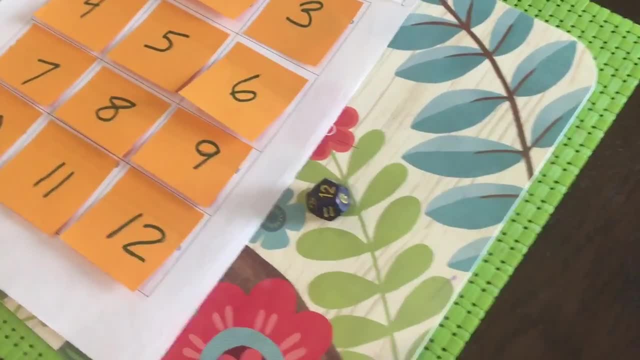 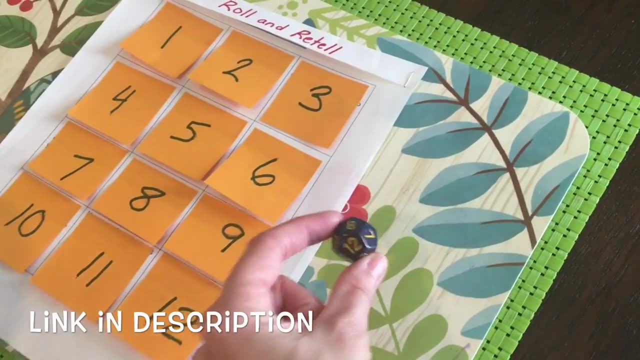 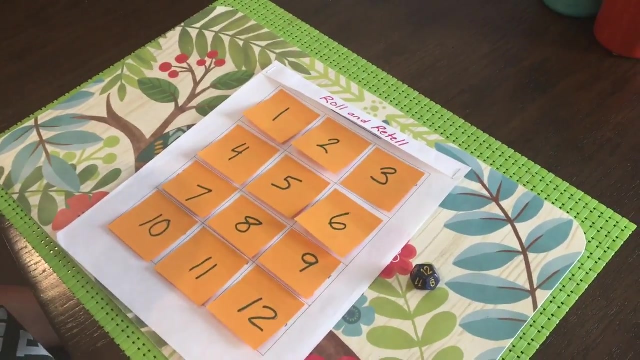 And Then you can get a die. We actually have a twelve-sided die here. You can get these off Amazon. You can also just use a six-sided die if you want it to be out of something you already have in your home. So what we're going to do is Wyatt is going to roll the die here. 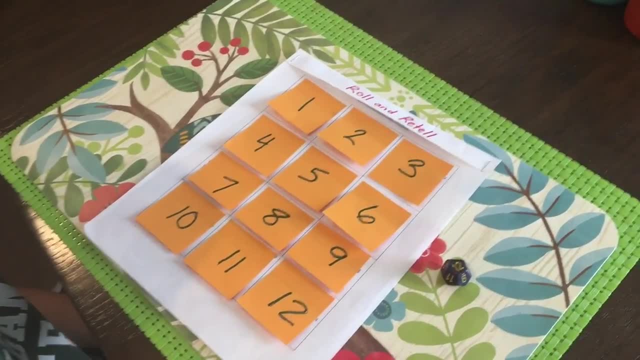 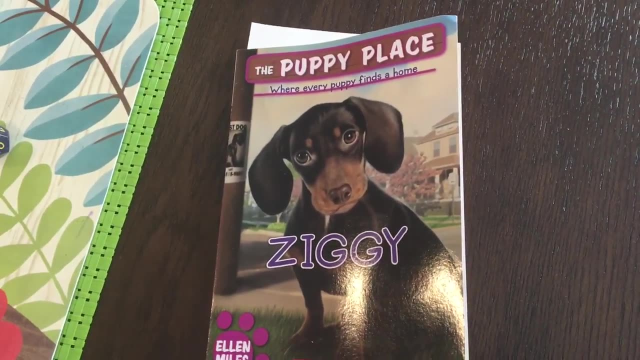 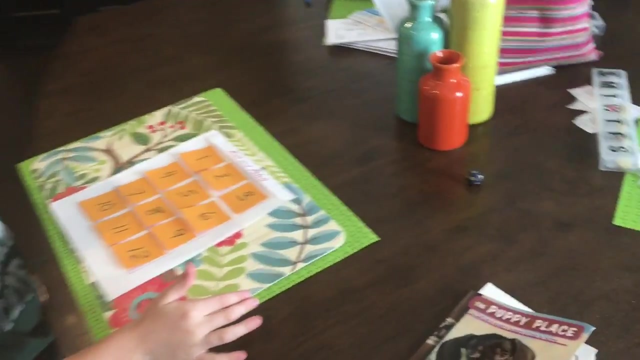 And then that number he will uncover and he'll answer the question. from what he just read Today, he read: The Puppy Place Ziggy By Eric, By Ellen Miles. Alright, Wyatt, go ahead and roll. What number did you get, honey? 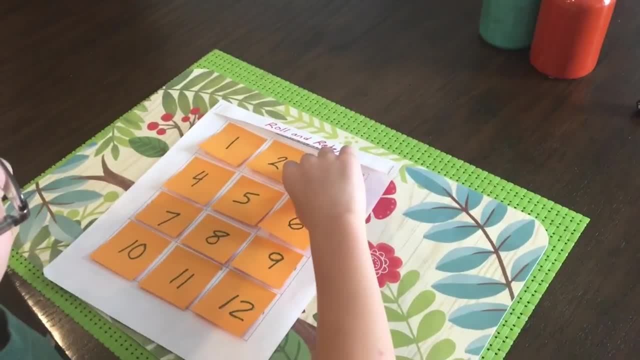 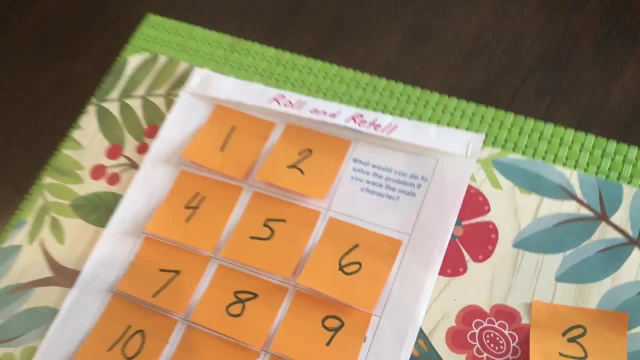 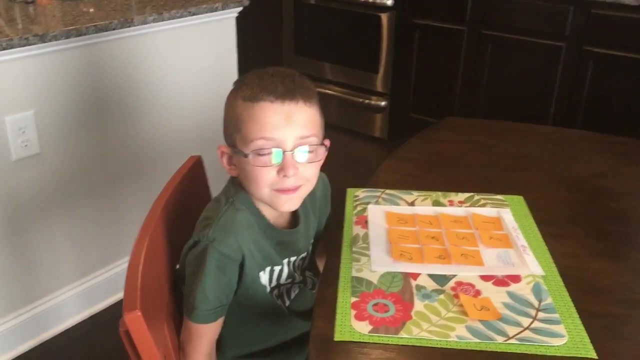 Three, Three. Go ahead and uncover three's question. Read it for us, honey. What would you do to solve the problem if you were the main character? Now, you had already told me that the main characters were Lizzie and Charles. Yes, 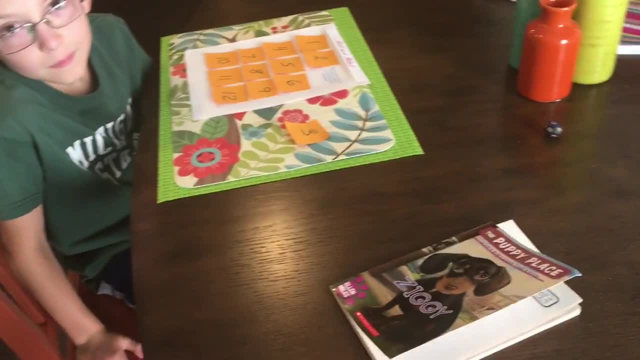 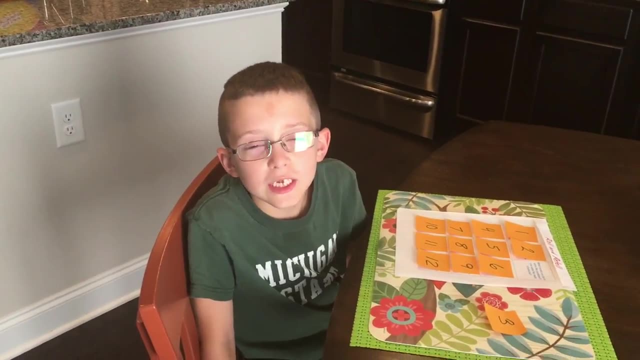 So what would you do if you were them to solve the problem of the lost Ziggy? I think, because they were a foster family, that they should take the puppy and foster him. Okay, And that's a good way to take care of a dog. 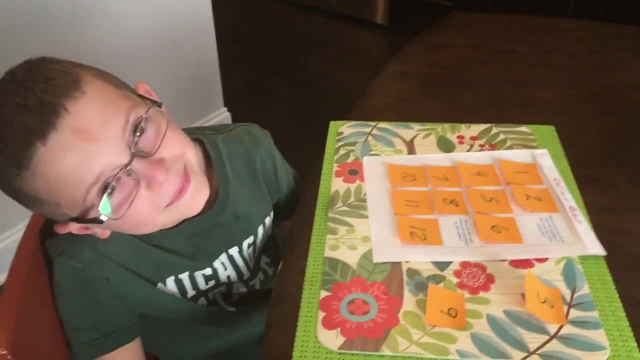 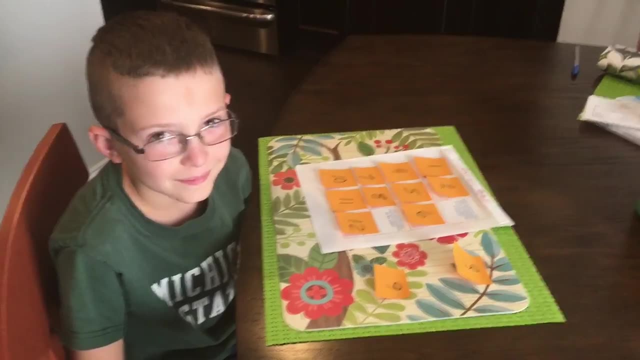 Until somebody else can keep him forever. Do you think it makes answering the questions a little more fun instead of just writing them down or just answering them one by one? Way more fun, Way more fun, Cool. Well, let's start the next one. 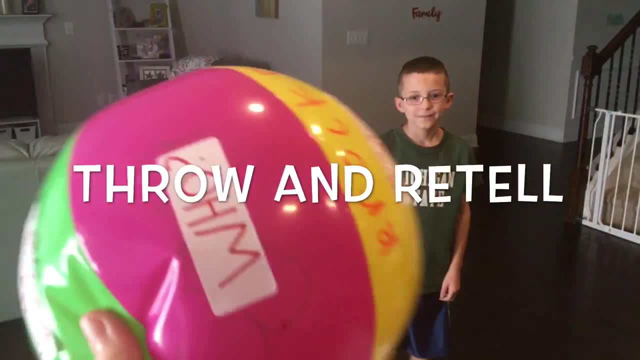 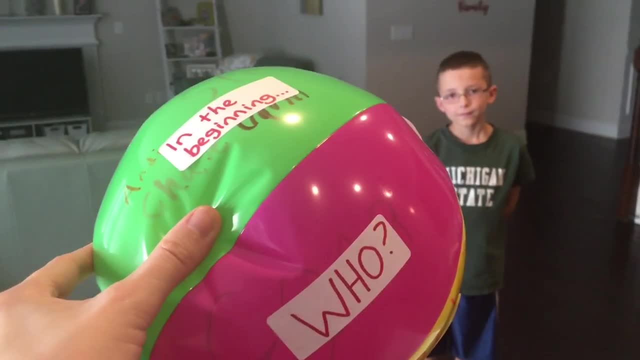 The next reading comprehension game is using a beach ball, And this is for your more active kids, If you want to give them something to do after school that will really get them moving and keep them engaged. I just took an ordinary beach ball from the dollar store. 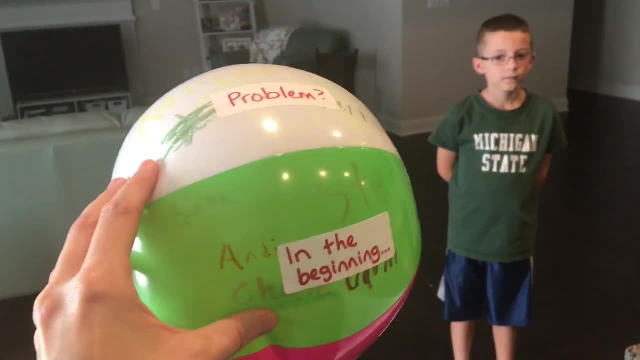 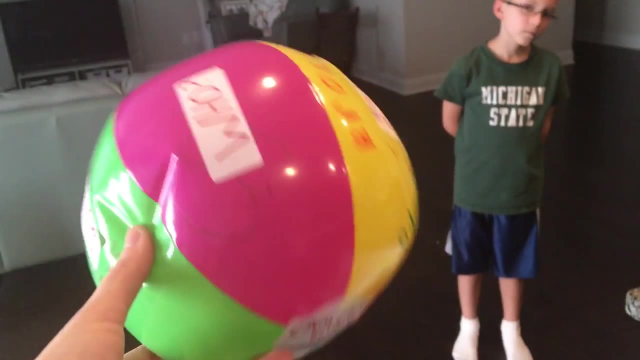 My son had one with a couple of his friends' names all over it. I just put labels on it for the time being. They say questions like: who in the beginning? What was the problem? There's even questions on the end that say: 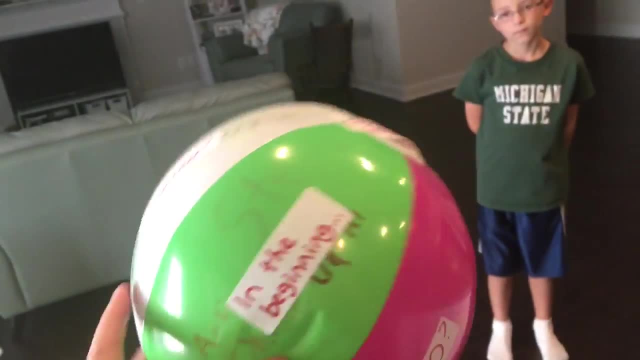 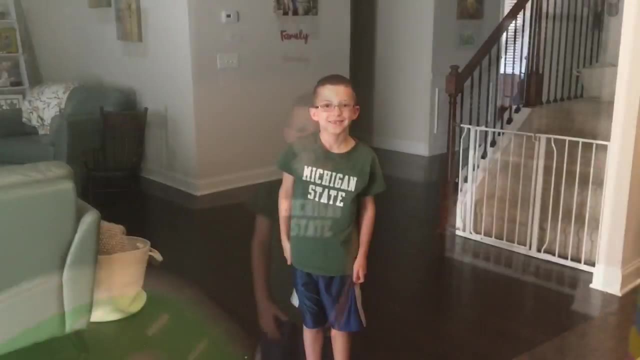 What was your favorite part and why? And I'm going to throw this to Wyatt and he's going to catch it And whatever his right hand touches, that is what he's going to answer. Alright, Wyatt, are you ready to catch? Yeah, Here we go. 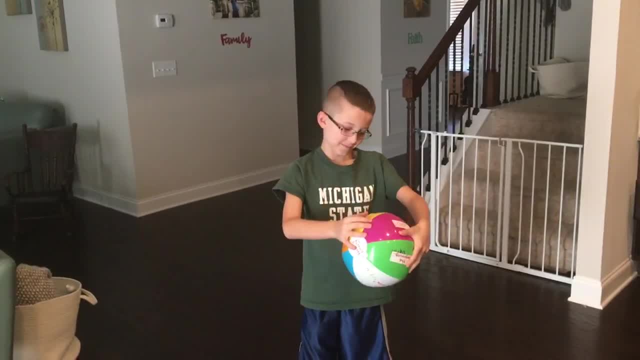 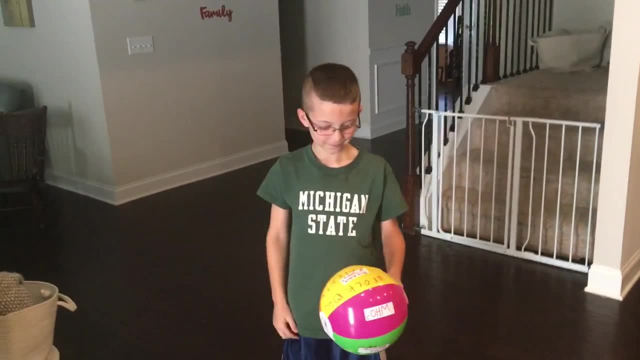 What is your right hand touching A big event of story? Alright, what was the big event of the chapter that you read today? And I do want to point out, moms and dads, that if you're only reading a chapter a day, 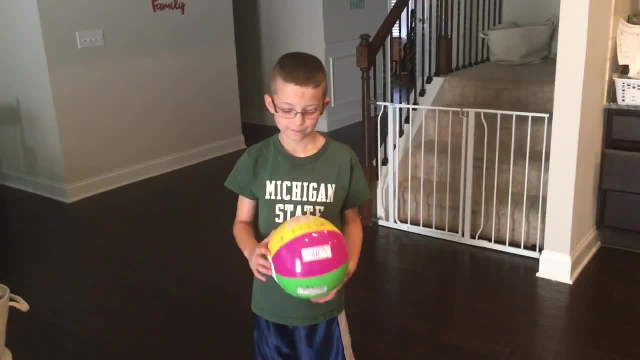 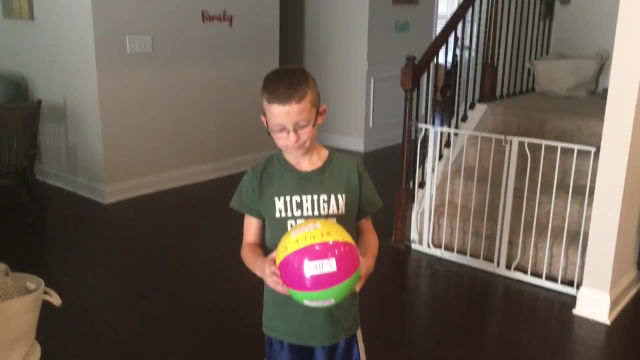 then this would be the big event of that chapter. You can also do it if they're reading an entire story to you. Alright Wyatt, what was the big event of the chapter you read today about Ziggy? I guess it was like the dog show. 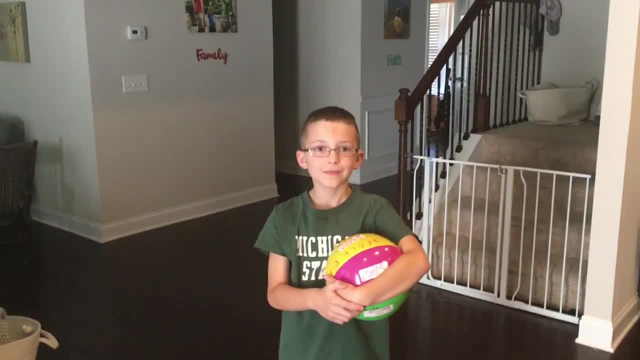 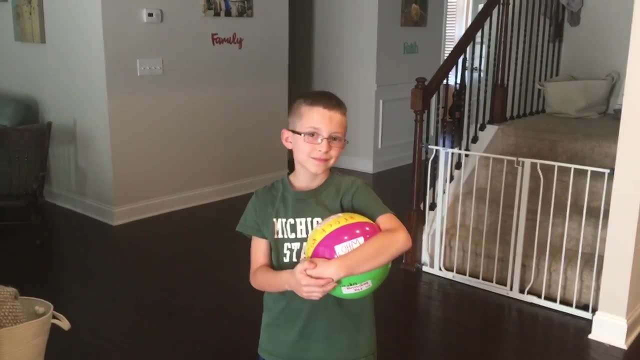 There was a dog show. Is that how they found Ziggy? Yes, Okay, so that's how it starts the story, because we're finding Ziggy, And Ziggy is an important part of the story because he needs a new friend, So he needs to have a new friend. 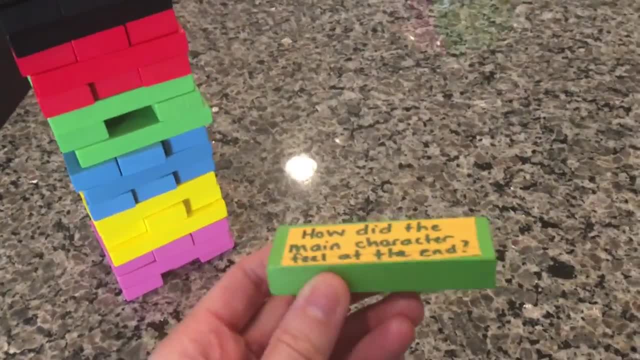 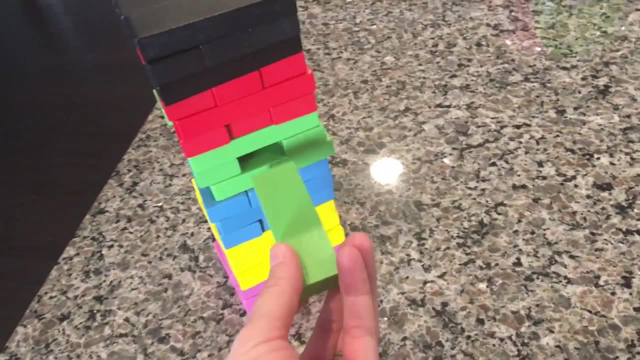 Right, he's a big, big fan of new friends And he came to know a new friend, So he's a big fan of the new friends and he's actually trying to get a new friend in the house And he's going to be able to give a new friend some love and affection. 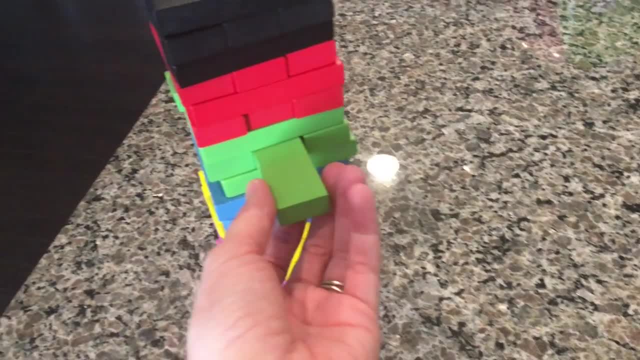 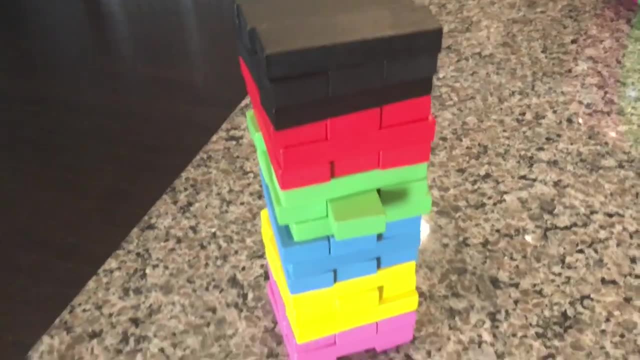 Alright, Wyatt, what are you going to do? I'm going to take the kids and I'm going to put them in the new building. Okay, All right. so it's going to be a very big event. That's what we're going to do. 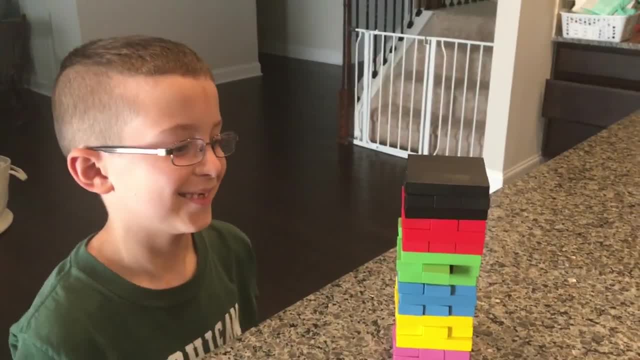 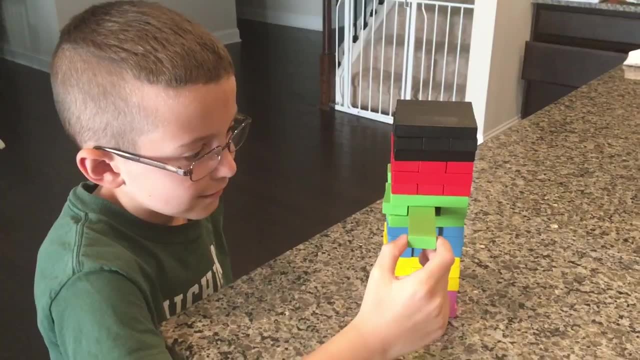 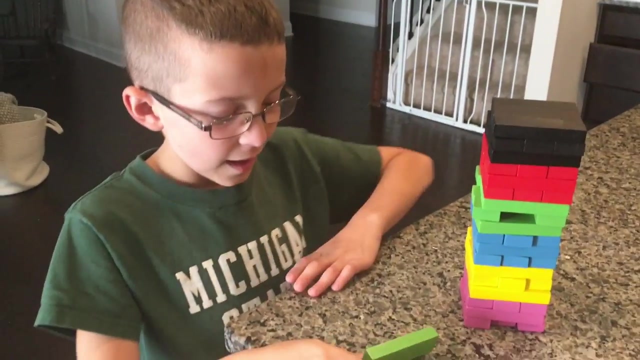 Because we've already talked a little bit about the 21st century And we're going to be doing that in the next chapter. see if we can do it without breaking the tower. nicely done. what is the comprehension question, honey? how did the main character feel at the end? so at the 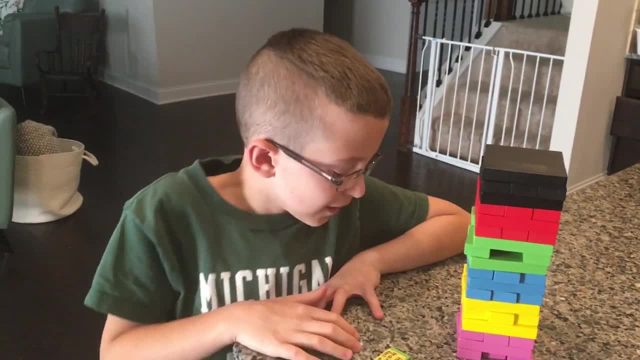 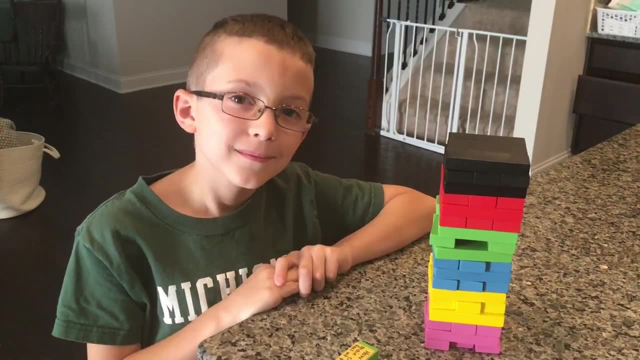 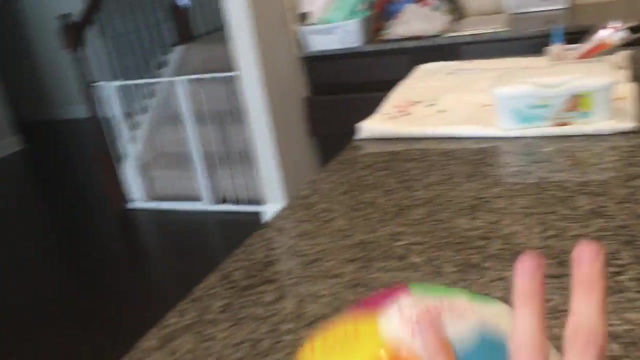 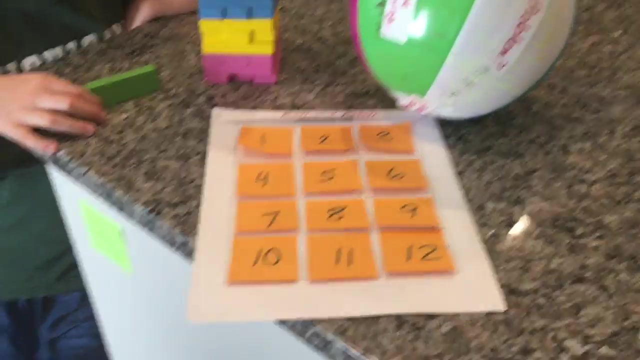 end of the first chapter. Wyatt, how did Lizzie feel? Lizzie felt happy to go see the pugs and ring too, because it was part of the dog show. yes, so out of this game, the throwing the comprehension ball and the roll and retail, out of all three.